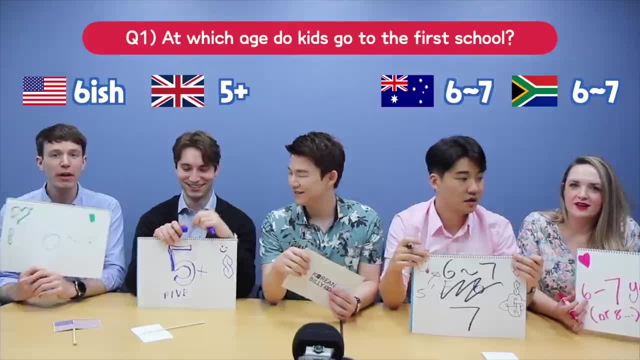 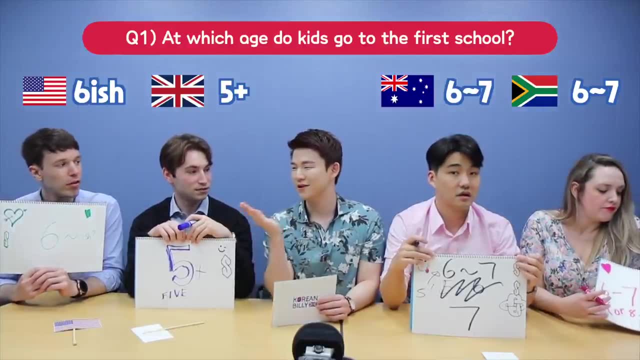 I believe so. Okay, His parents were very young. I'm pretty sure it's around 6 years old, I think it's 6. It looks like 6.. So this is kind of the average. Yeah, and UK 5?? 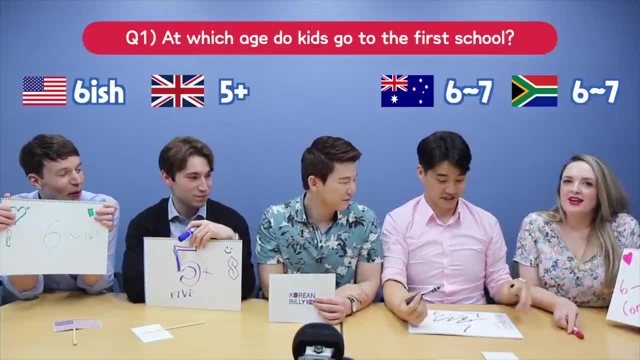 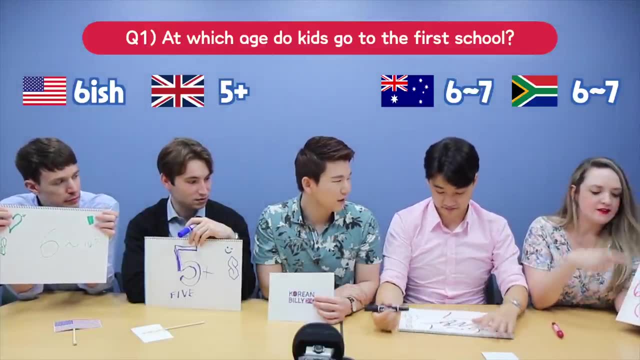 5,, 6,, 7.. Mine is generally it's 7.. Okay, Sometimes parents will send the children to school a little earlier. then it's 6.. For people who are born in December, the parents tend to keep them back a year because our school systems are kind of weird. 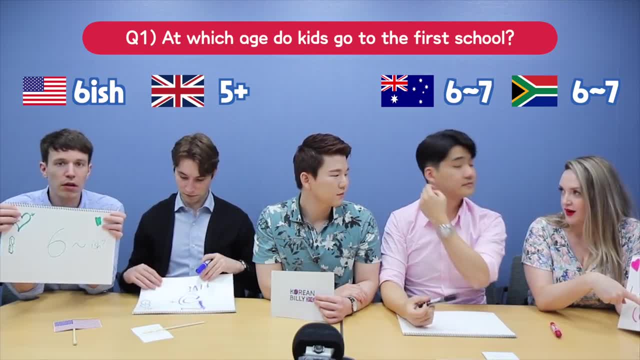 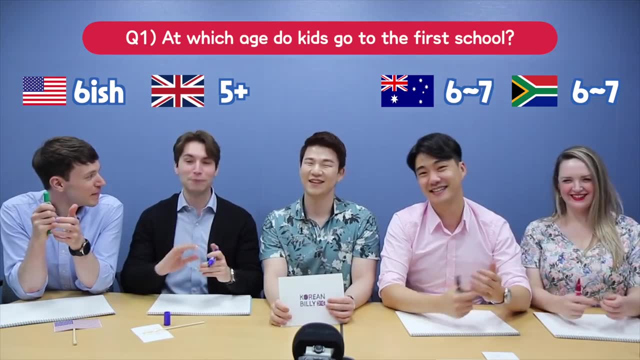 I was 8 and my best friend was also. We were 8 when we started grade 1. So in the UK, like kids start their education very early then, I guess, so I'm sure it's different all over the UK. 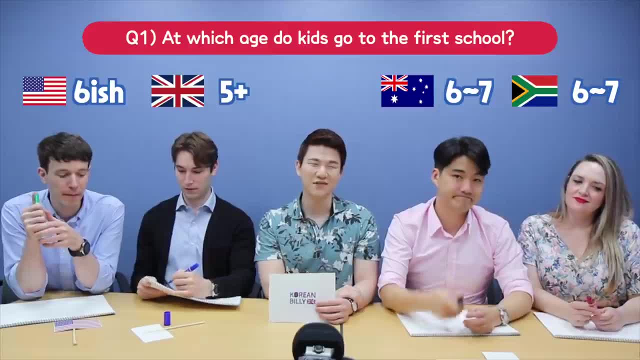 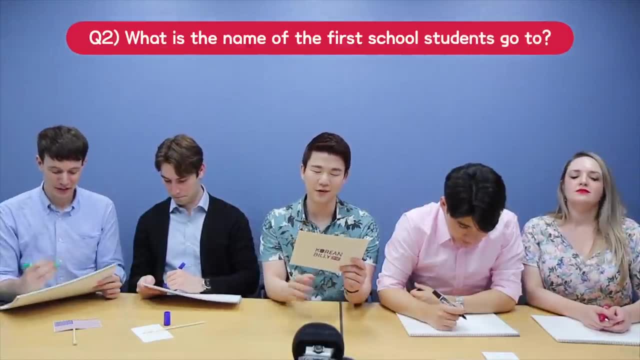 Yeah, It's actually different in Australia, like state to state. It may differ even within those countries. Yeah, that's true. Okay, the next question: What is the name of the first school which students go to? 3,, 2,, 1.. 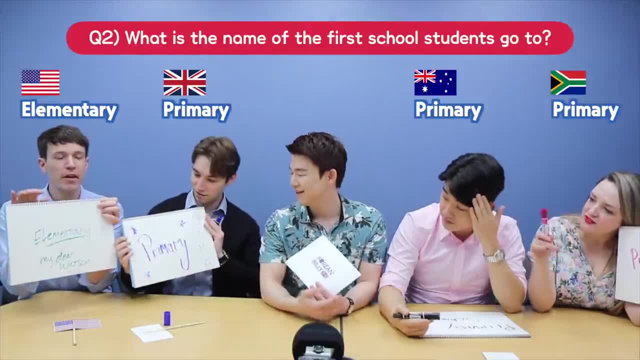 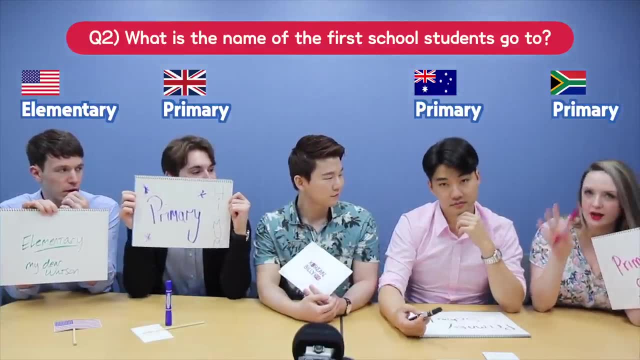 Elementary, primary, primary, primary. I have to say, though of course this is only in English, We have other languages, and that would be something else- that I'm responding for English. For how many, How many years did you go to elementary school? 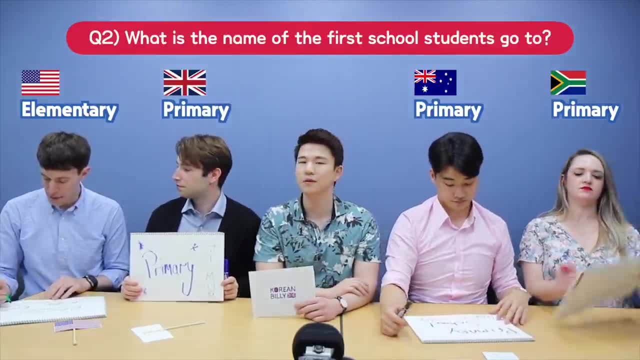 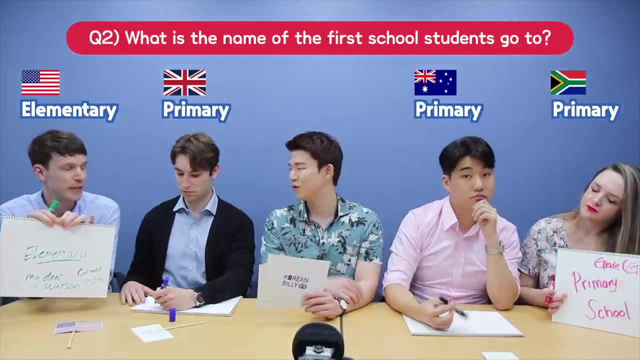 I think it's the same. It's well, it depends Like. I think you can do it early, So it's like 1 through, let's say like 5 to around 6 ish. What about you guys? What about elementary school? 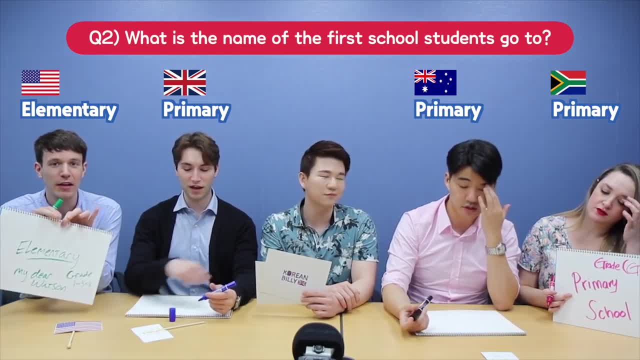 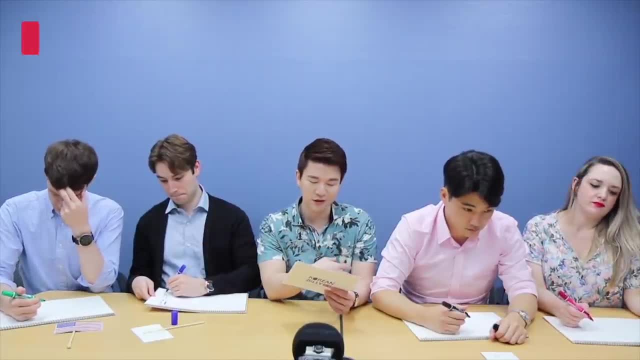 Have you heard of it? No, Only in America, Oh, I know about it, But yeah, only in America. American drama, Yeah, All right. So from the first school, elementary school and primary school- for how many years do students go to school until going to a university? 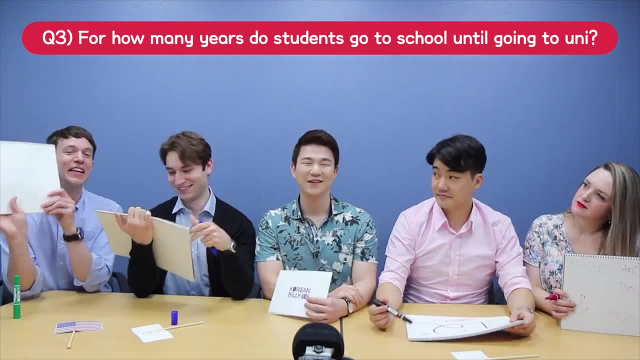 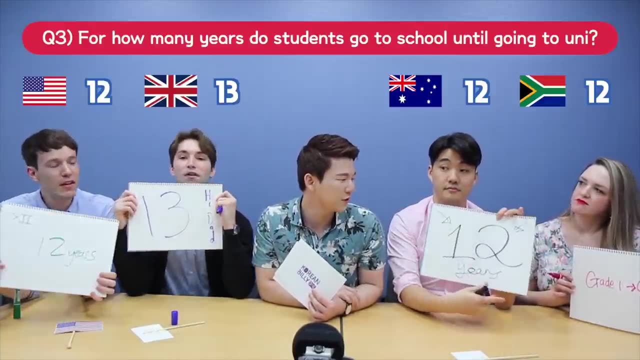 In your country, From elementary to graduation, high school. Yeah, Okay, So 3,, 2,, 1. 12,, UK 13,, 12 and from grade 1 to grade 12.. They have in the past few years, or a few years ago I think, they've added a preschool grade. 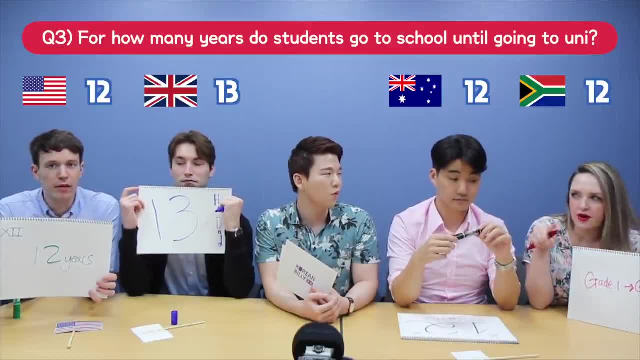 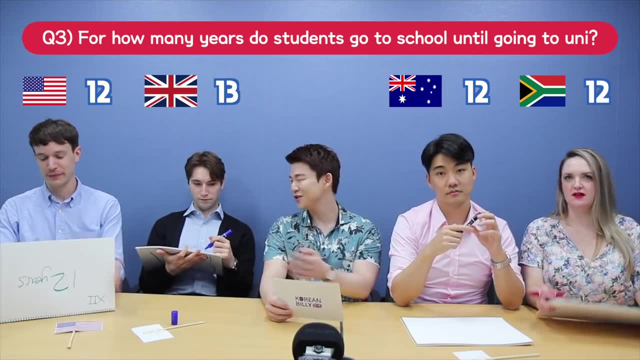 That's kind of like school. It's called grade R or grade 0. But when I was a child that wasn't a thing. We just had like nursery school and playgroup. Oh, that's true, Grade 0.. And British people study. one more year. 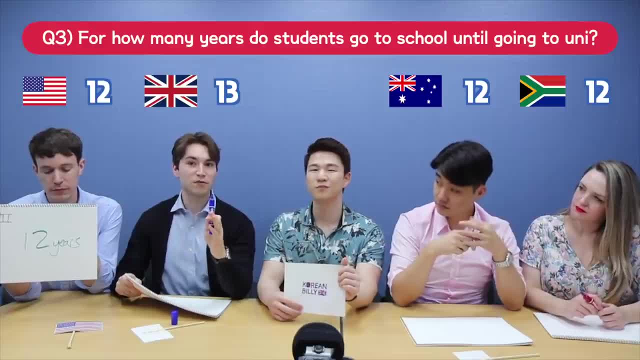 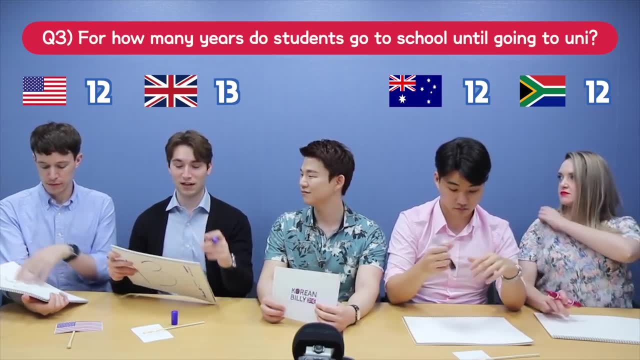 I think it is optional. You can start at 5 or 6.. But yeah, for me I'll start at 5.. Naturally, because you start earlier. Yeah, Start to go to school earlier. Yeah, I don't know why. 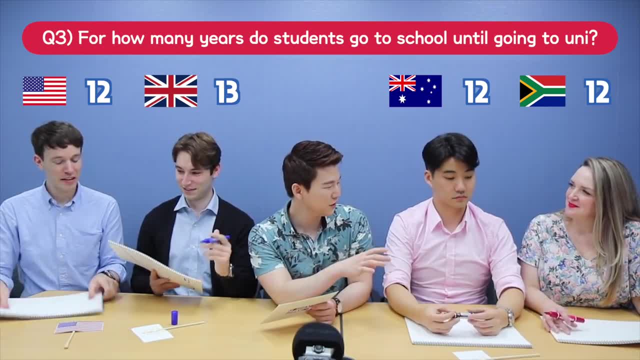 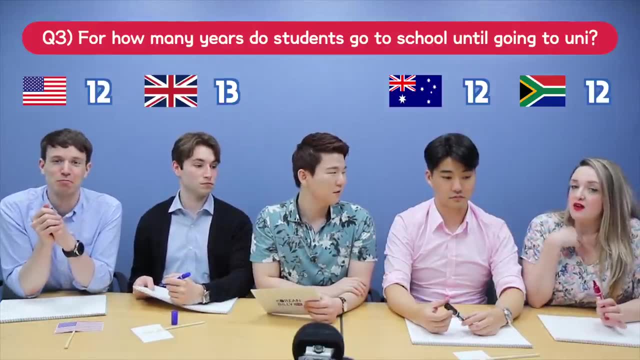 It didn't make me any smarter In South Africa. don't you use like year 1 or year 2?? Do you use the word grade? Usually? grades You too? Yeah, When I was like when I just started primary school, it was sub A and sub B for grade 1 and grade 2.. 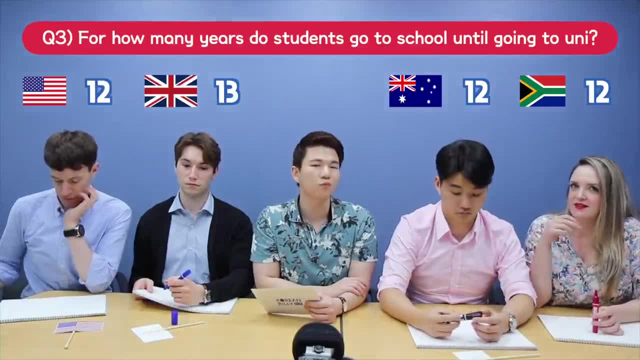 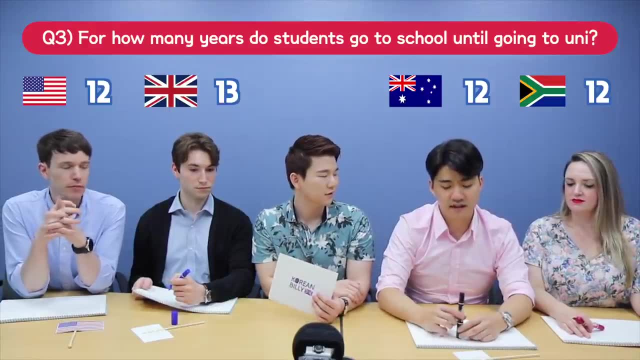 But then they changed the system and everything is grades Yes, until grade 12. And it seems like Australian one is kind of following the UK one. Yeah, there's a lot of fault. I believe that, like I have heard of grade 1 and grade 2.. 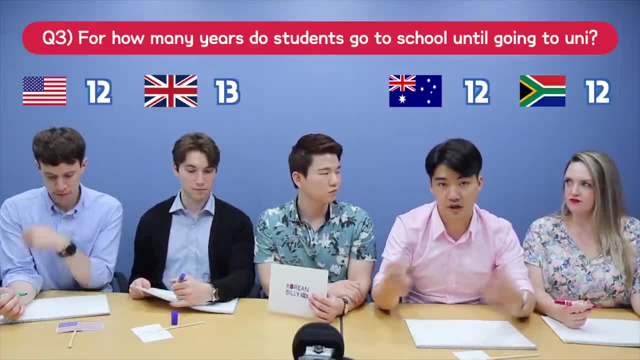 I'm not saying that Australians don't use that, because I have heard it, But I always grew up year 1, year 2.. And in the US, after elementary school, what schools are there? Is it middle school and high school? 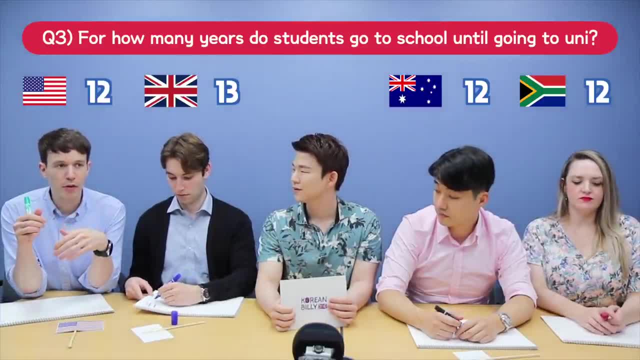 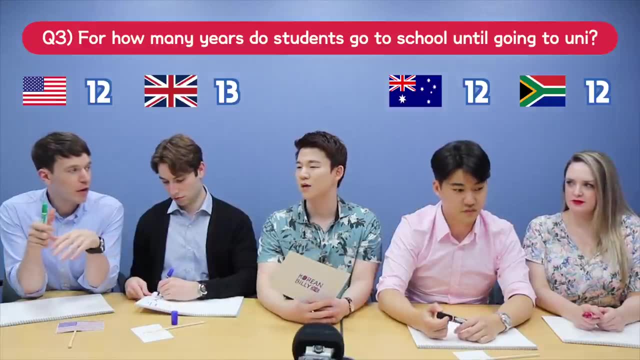 So elementary, middle, high, But there's also something called junior high that can be split. Junior and high can be put together and there's no middle Wow. So there's a few different ones and it really is school dependent, Even public school dependent. 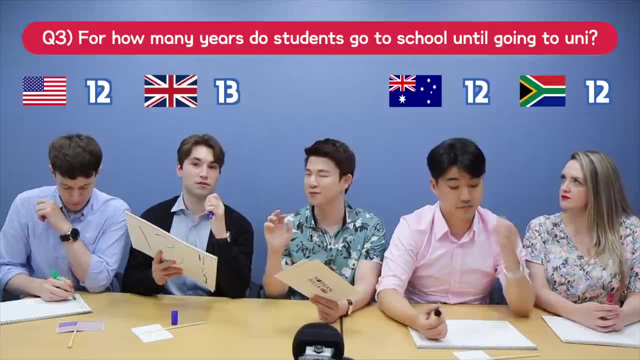 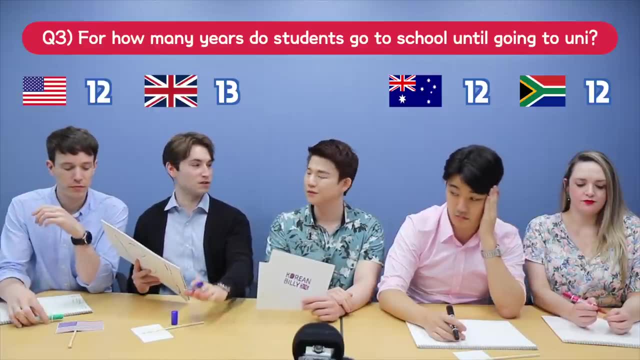 What about in the UK? after primary school, Do you go to something called middle school? No, I do believe there are some middle schools in the UK. My stepbrother went to a middle school, But the typical system is primary, secondary. 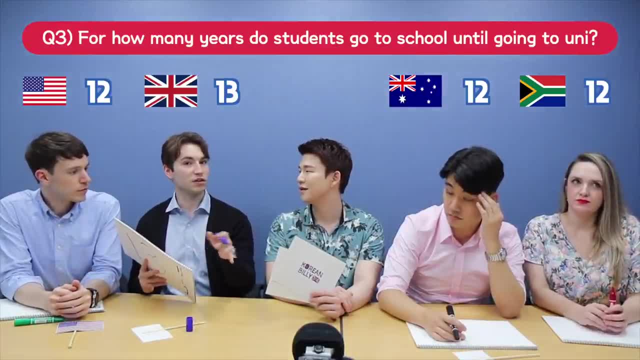 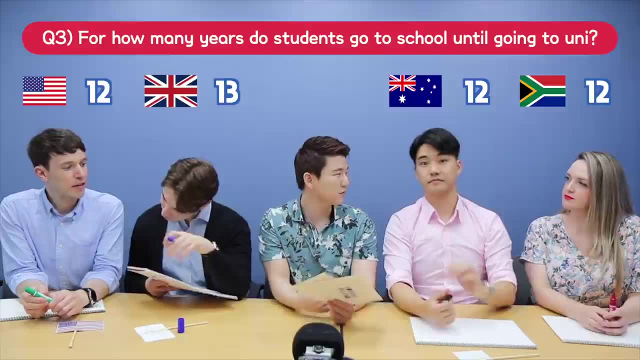 And then you can go to college if you want, or you can stay on a kind of higher education And then university. So we have a few routes you can take. What about in Australia? Is it also primary and secondary? Yeah, yeah. 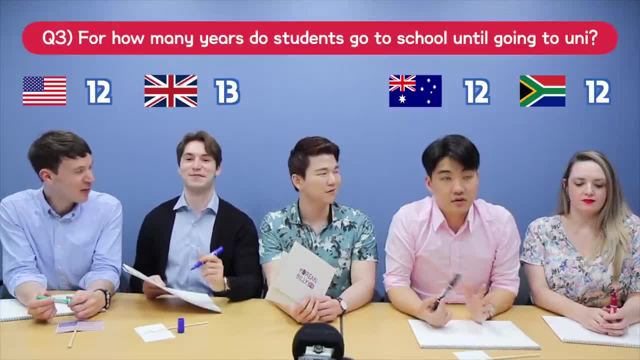 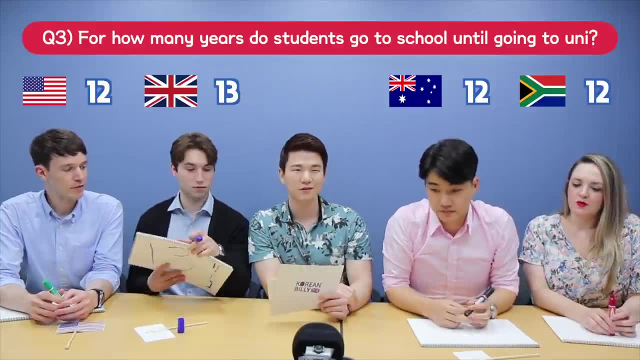 Basically from when I went to school, it was like year or grade 1 to grade 7 for primary, And then it was for me grade 8 to grade 12 for high school- Also primary and high school- and also high school is also known as secondary school. 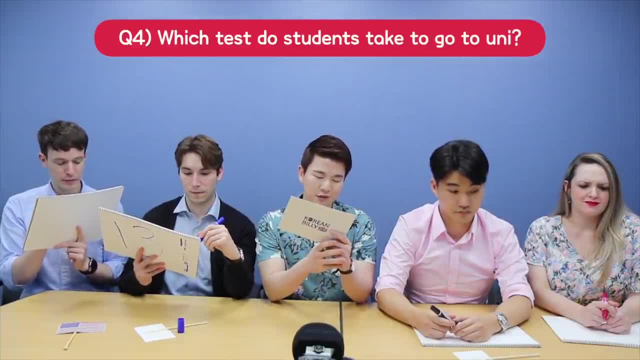 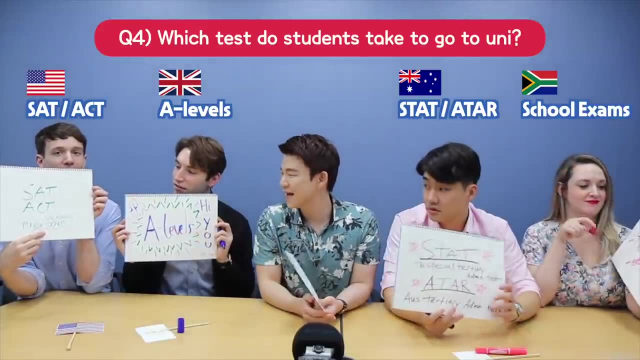 Next one: Which test do students take to go to university? Don't ask me that question. So 3,, 2,, 1. In the US it's called SAT SAT, Or that's why it's probably called the Korean SAT. 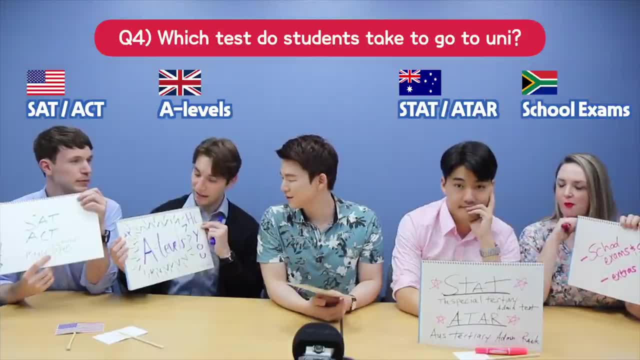 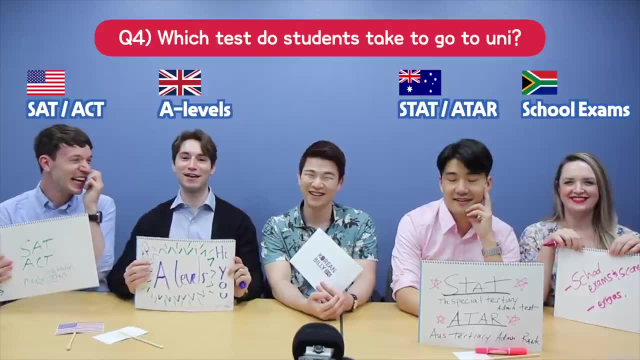 Or ACT, ACT. Pretty sure I got those correct. A-levels, A-levels. Don't ask me what it stands for. Did you take the B-levels? I took the S-levels, fam. So yeah, A-levels. 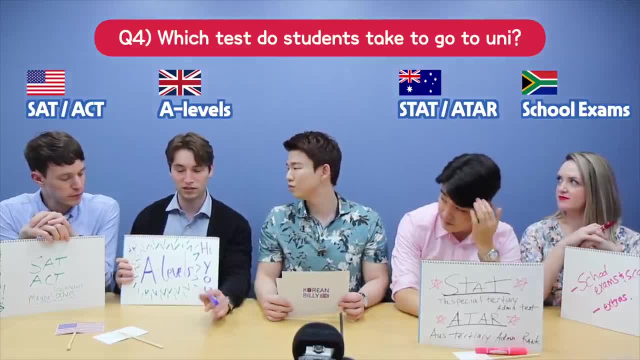 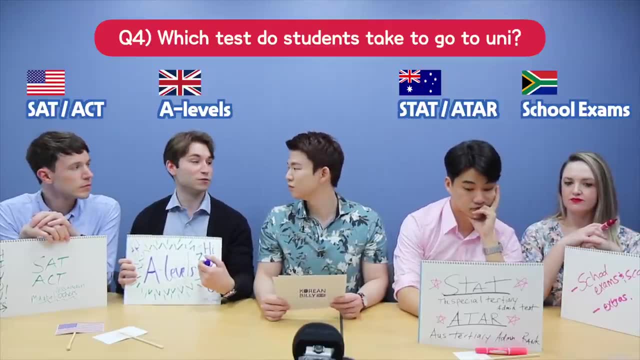 But we have a kind of a system where, from age 11 or 12 to 16, you're preparing for your GCSEs, which is an exam to kind of get into your A-levels. Wow, that sounds complicated, Okay. so first things first. I actually didn't do this test at all. 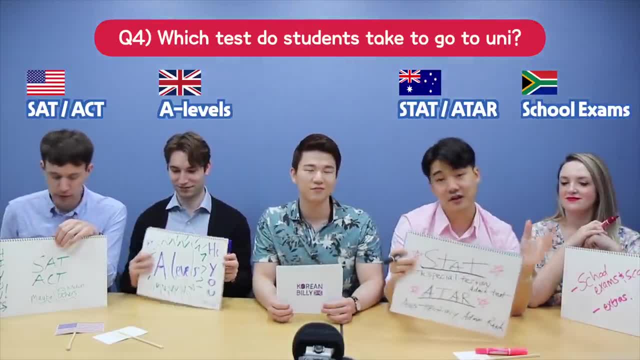 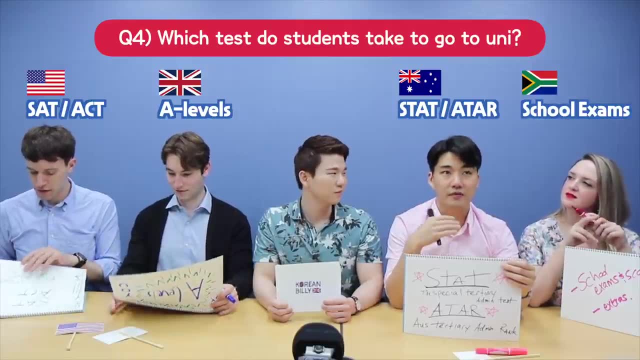 I went a different way to go to university. I went through TAFE in Queensland, which is kind of like the Well. originally my plan was never to go to university, I just wanted to get just a normal job and do it that way. 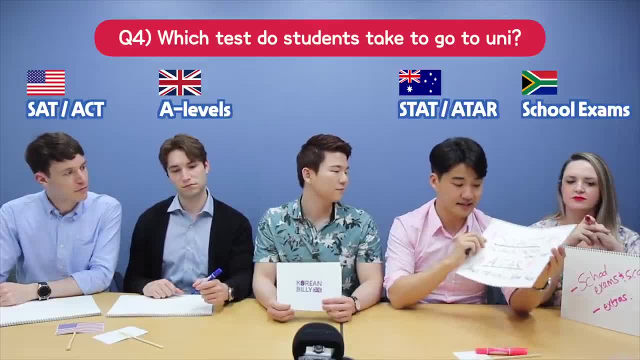 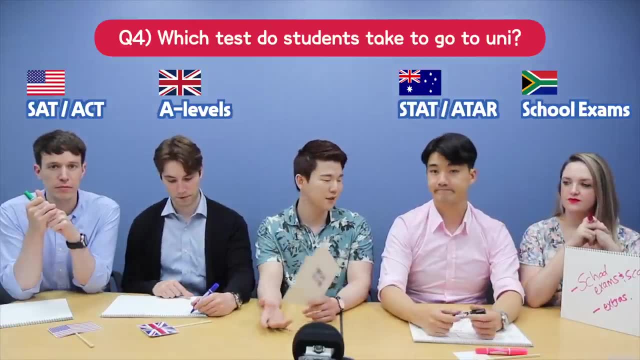 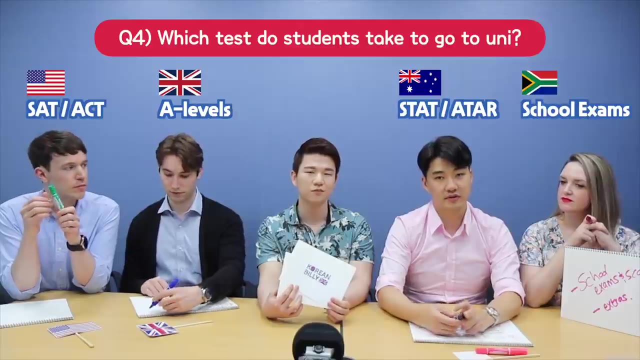 However, from what I remember, it's the STAT or STAT tests, or the ATR tests. Wow, ATAR, ATAR, STAT. It might depend on states. right, It would also depend on states as well, Like I think, TAFE is a popular way of going through for most states as well. 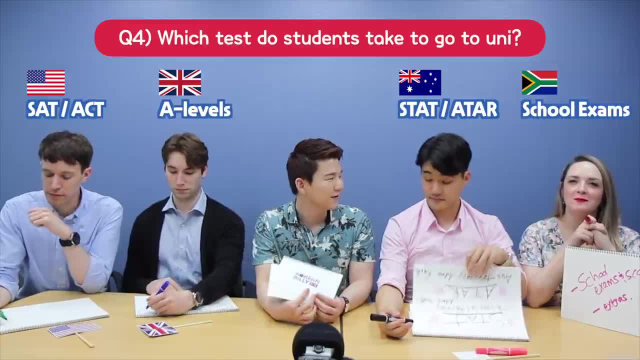 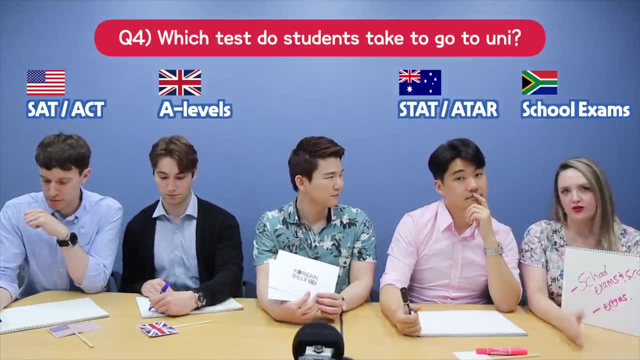 But yeah, that's what I did. I absolutely can't remember, Okay, And I'm not 100% sure, but I can say it's a final exam. So when you finish grade 12, you write a final year exam, but the universities actually start. 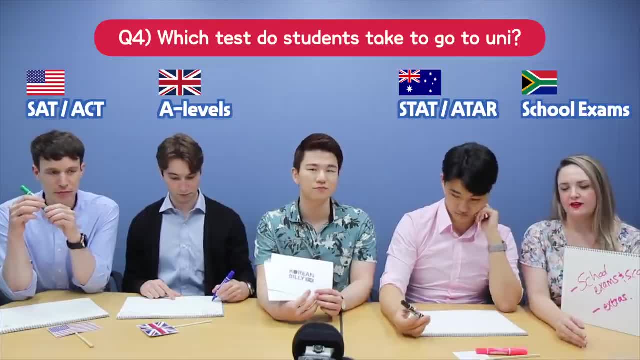 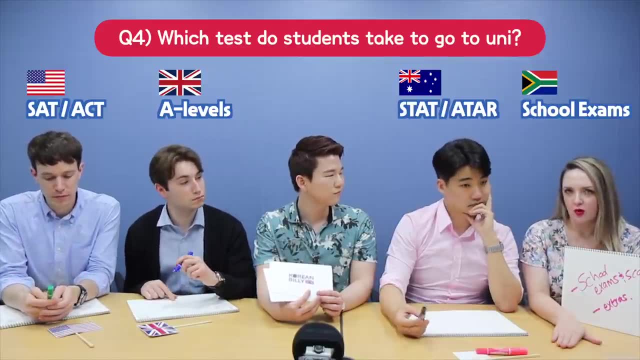 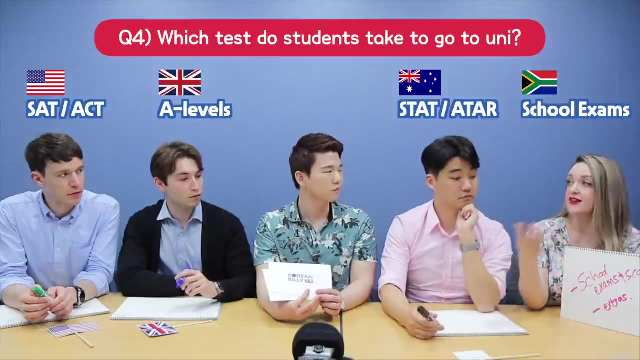 looking at results earlier because we apply earlier, So they consider end of grade 11 results as well. We then hand in the scores to the universities. when you apply- I think some of the majors or the degrees- you might have to write another test. but 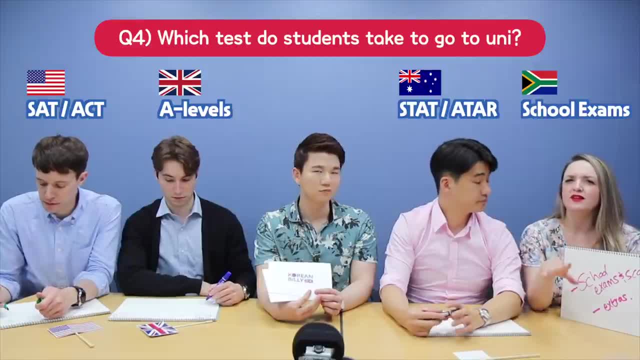 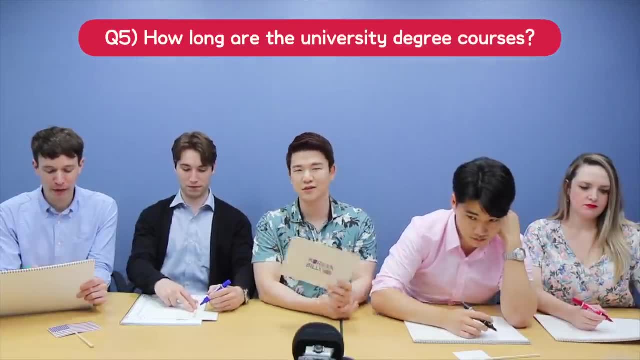 what I studied. it wasn't necessary If we call it something I honestly forgot. so South Africans, just help me out here. Next one: How long are the university degree courses in your country? So three, two, one, Three, two, one. 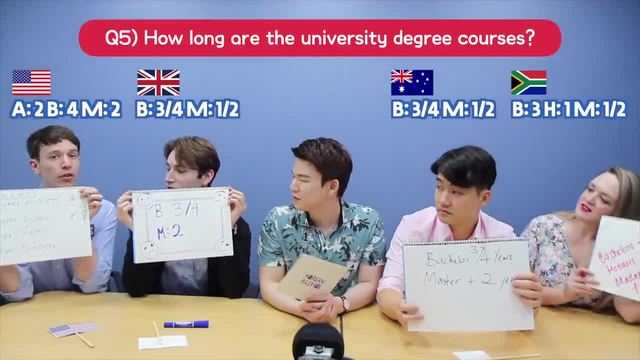 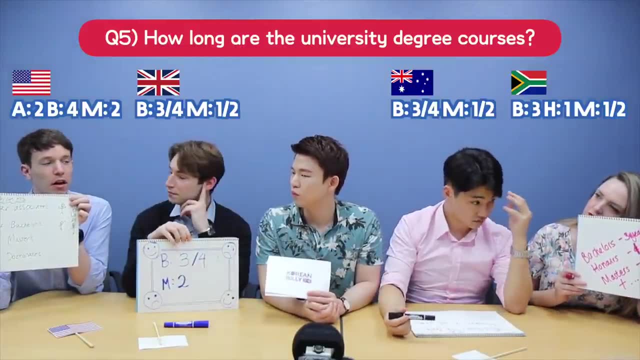 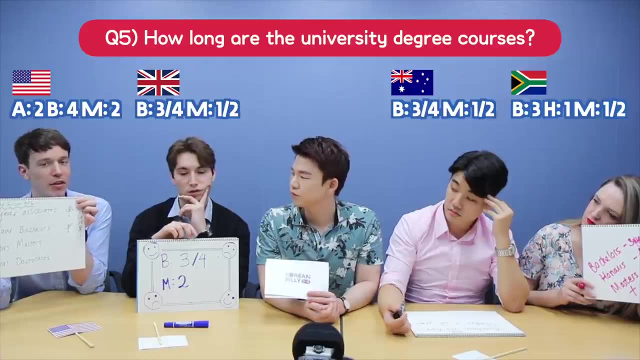 That's really complicated. These are total years from high school. Wow. Two years for associates- Not all colleges have associates degrees. Four years from high school for bachelors. Six-ish for your masters, then around seven to ten-ish. Ten is on the real high end. 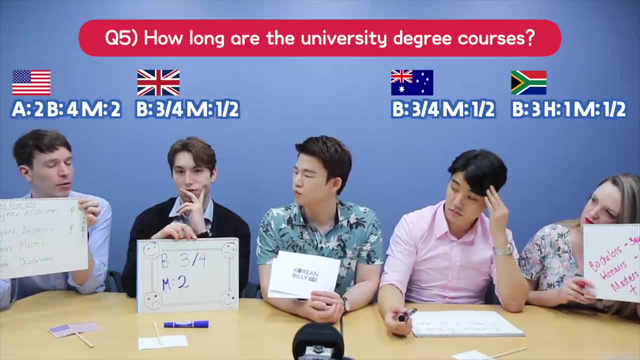 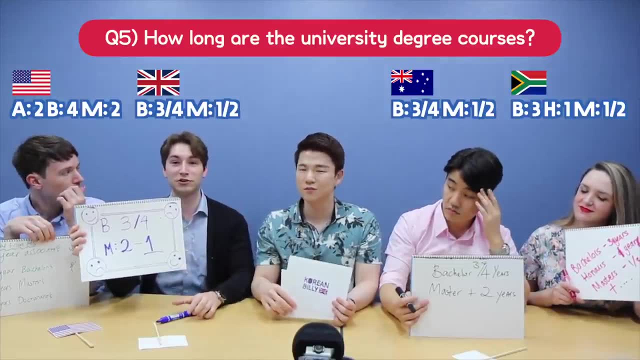 So I'd say seven to nine, seven to eight for your doctorates. Bachelor typically takes three years. There are some that take four. It does depend on your major, your degree. And then masters was typically one year. I'm sure some places were two. 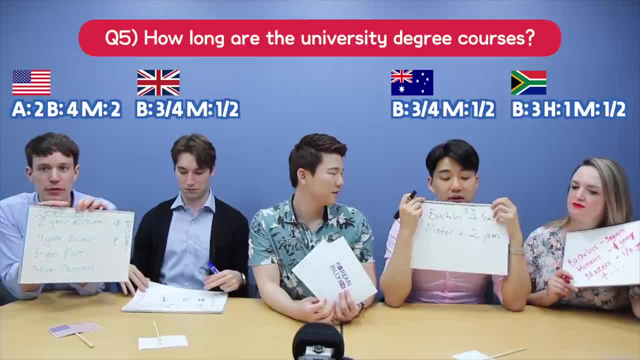 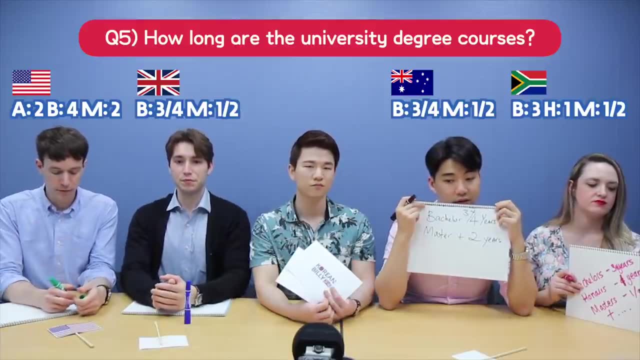 I think it really depends on like, where, Like, as an example, my degree was three and a half years, Three and a half. Three and a half years, You mean one more semester, Yeah, Masters? yeah, I guess it's like one to two years. 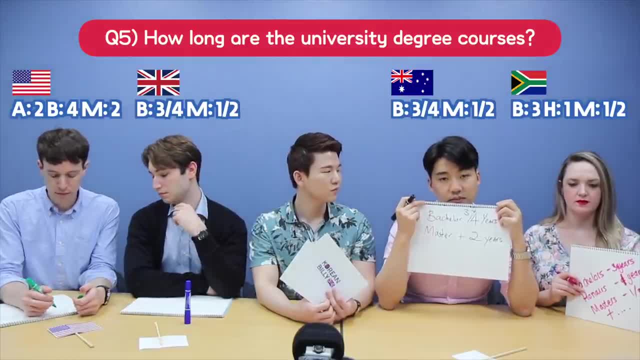 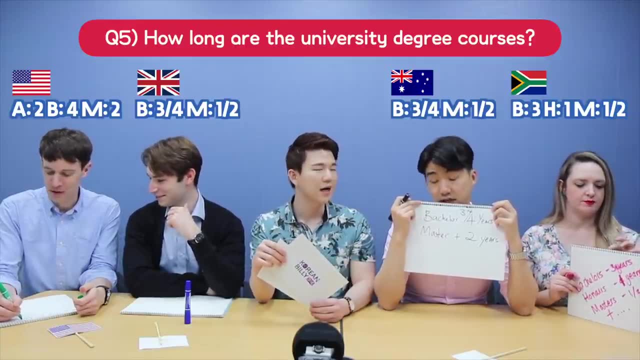 But then we also have double degrees as well. Double degrees also take a bit longer. Double majors, Yeah, You mean for double master's degrees, Double degrees, So you can get two bachelor's degrees, Two. So for most of them, or many of them, three years. 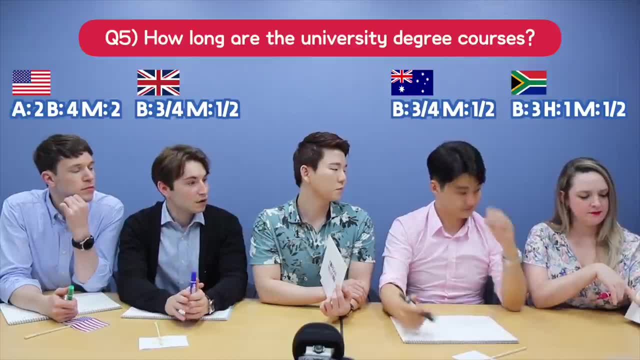 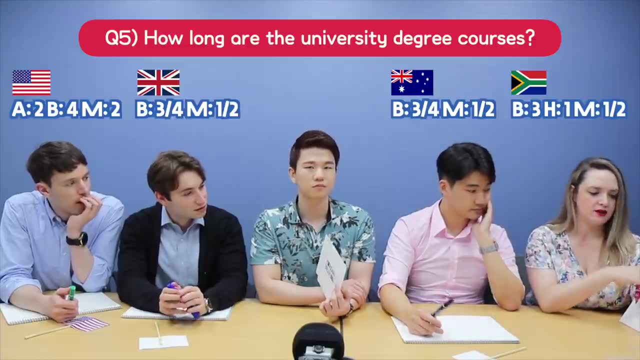 Then we have a year called an honors degree. Oh, we have that. That's an added year, That's a fourth year, So I went up to honors. Our normal bachelor's is the same as all of yours: It's three years. 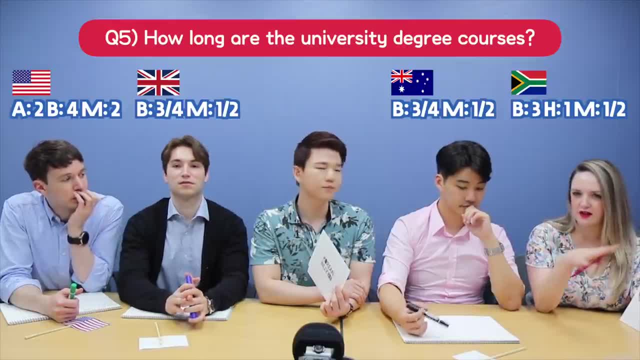 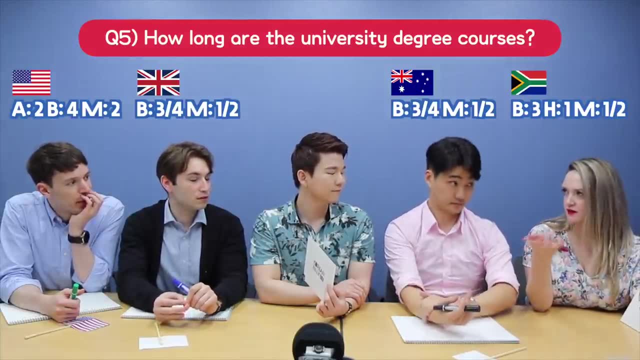 But I think some majors is longer, All right, So it depends, like theology and medicine and stuff like that. Then our master's it really depends. It's one to two years And of course you get your PhD, which is longer. 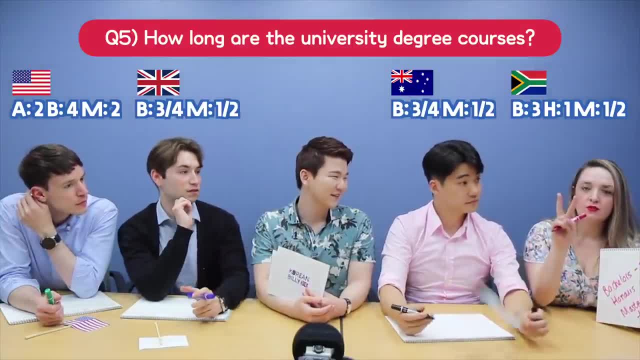 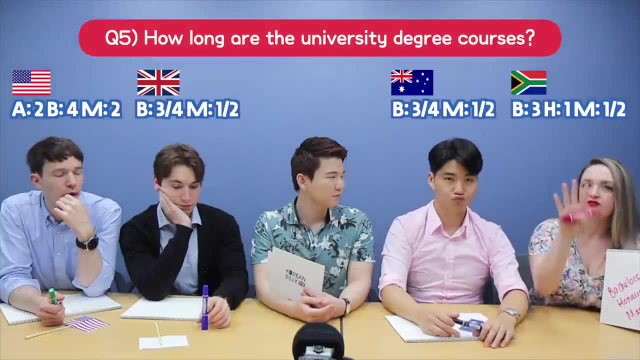 But we also have. we have other places that are not. they weren't universities, It's more like a college type of thing. Our college is not university And then you would have your degree after four years, not three years. I think American bachelor's is the longest one. 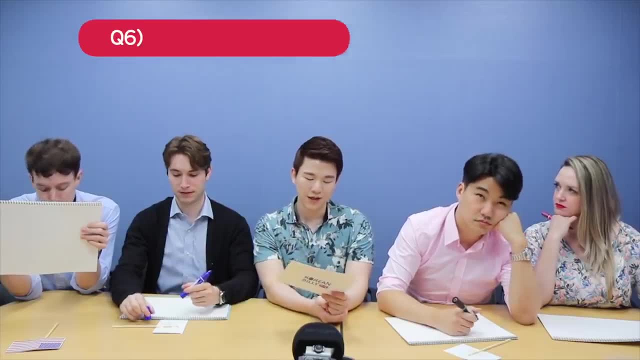 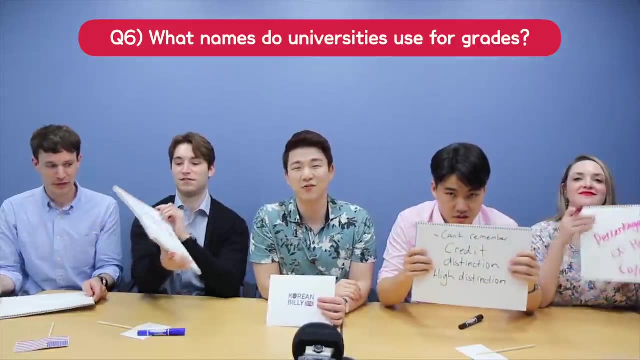 So is the Korean one. So what names do universities use for grades? Oh, okay, Okay, Three, two, one, Yes, All right, Very different. I think I answered wrong. I feel like we're not on the same page. 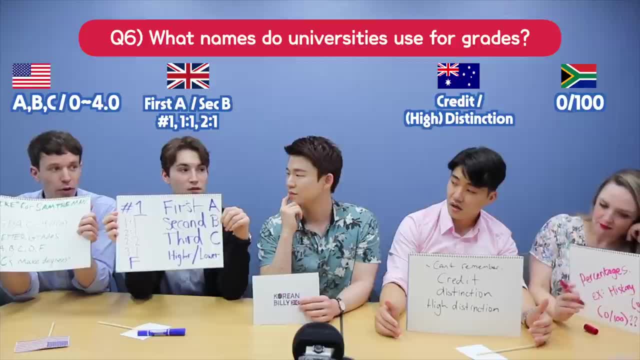 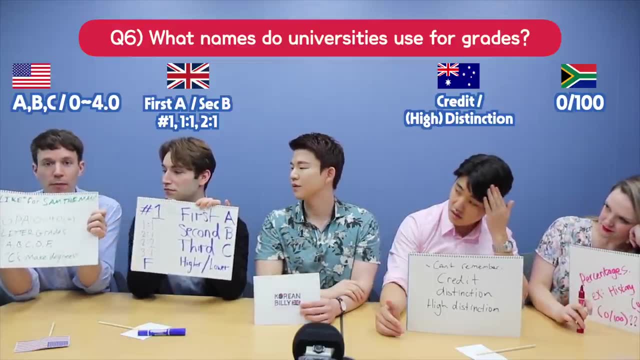 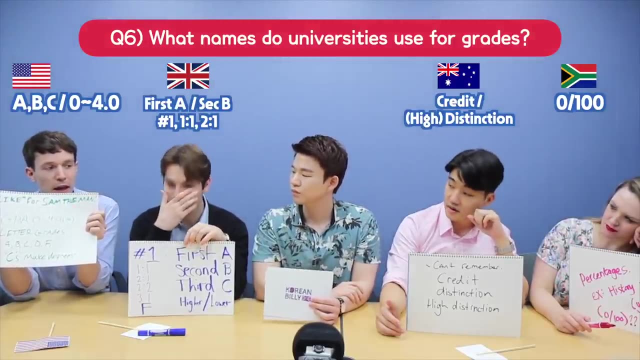 I think we're all misunderstood. So for each lesson you do and each class you do, you get a basic letter grade. Okay, But that basic letter grade will translate into something called GPA, grade point average. So at the end of the semester you will have a certain GPA at the end of your whole bachelor's. 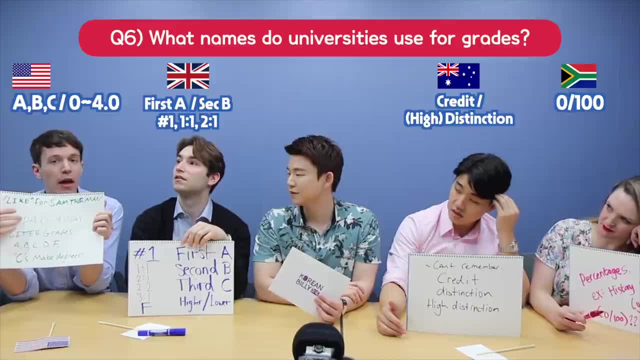 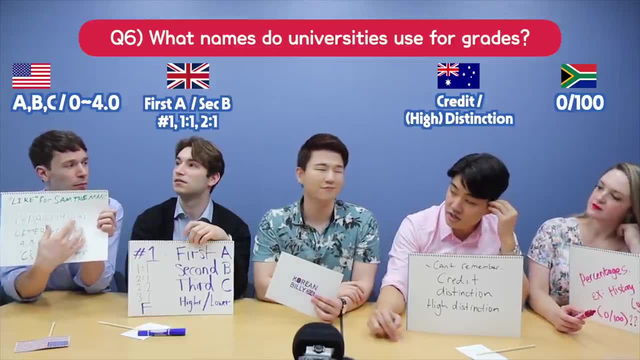 degree. So whatever you're doing, you will have a between a zero and a four point. I don't think anyone can actually get a zero. It might be 0.1 or just one. I know this GPA is also different from universities to universities as well. 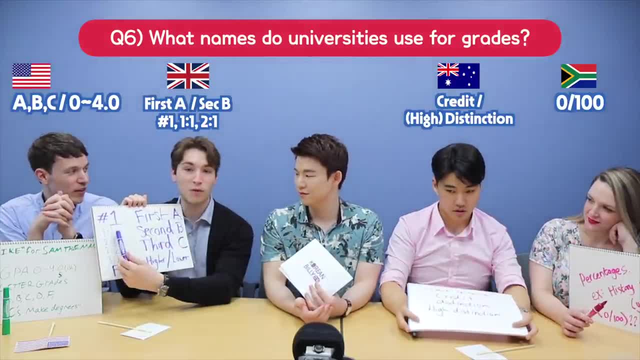 Is it? Yeah, I think so. Yeah, Okay, A first. we also call one one. There might be a one, two, I'm not, I really can't remember. It's like the highest grade, That's basically an eight. 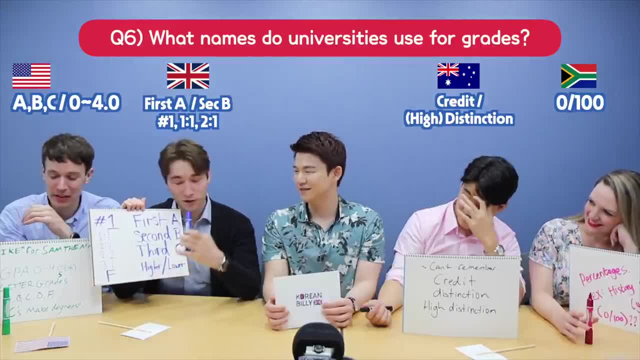 Basically Okay Generally, Then a second and then a third And then you fail. basically The grading system is so weird, At least in my uni, I'm not sure about other unis. So 60 to 70 was a second. 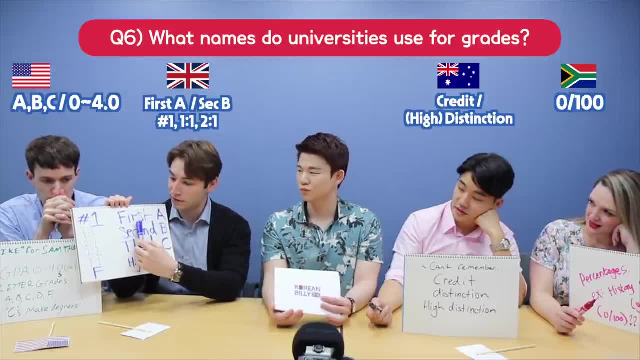 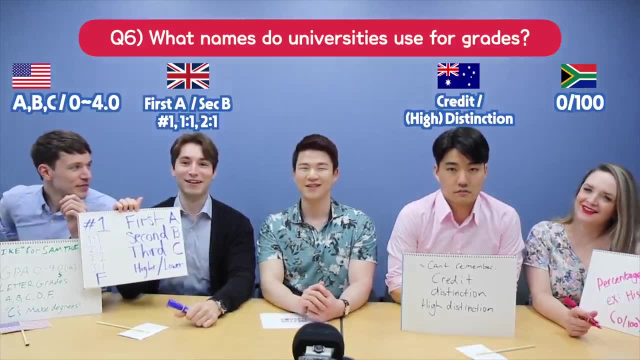 If you got 70 and above, it was a first. Oh, so that's like a distinction. Yeah, Yeah, Distinction. Yeah Yeah, We got 85.. Yeah, We have distinction. Oh my God, Can somebody like describe it in the comments? 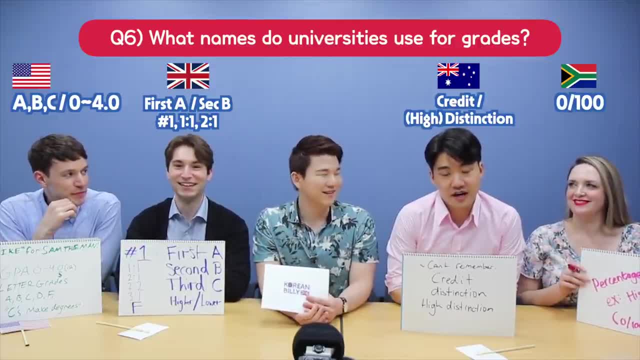 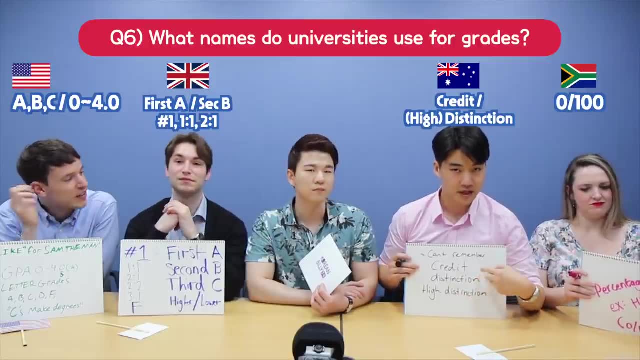 Yeah, Australian one Okay. So first off, I didn't care what I got, As long as I passed Amen. There's a standard which I can't remember, but I know above the standard was credit, Then there was distinction and then there was high distinction. 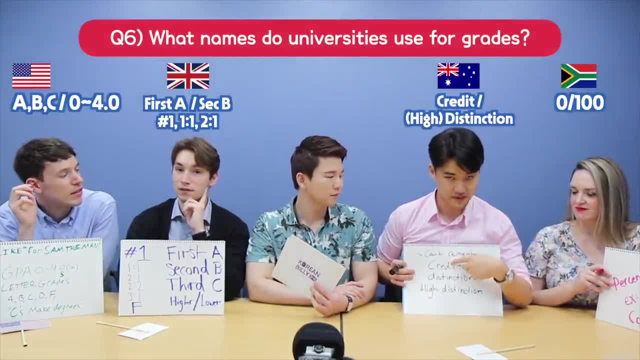 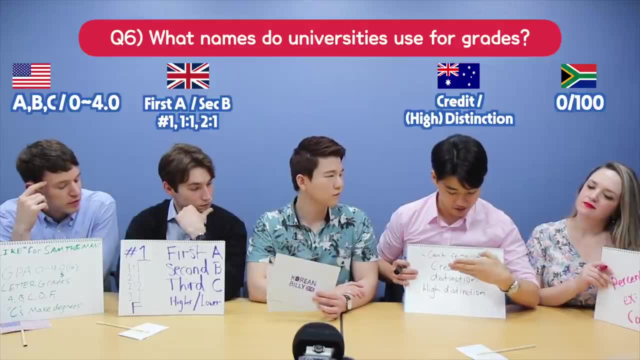 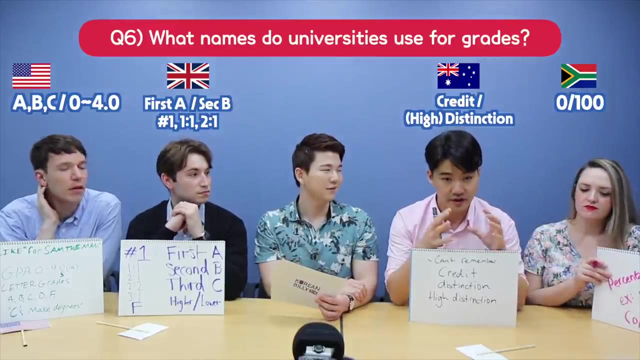 Off the top of my head, credit was between like 60 and 70% ish, And then I think it was distinction was like 70 to 80. And then this was obviously 80 above the high distinction. We also got a GPA at the end of each semester like an overall average, and then it added: 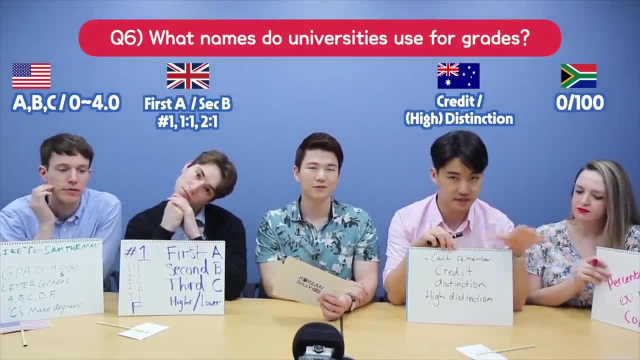 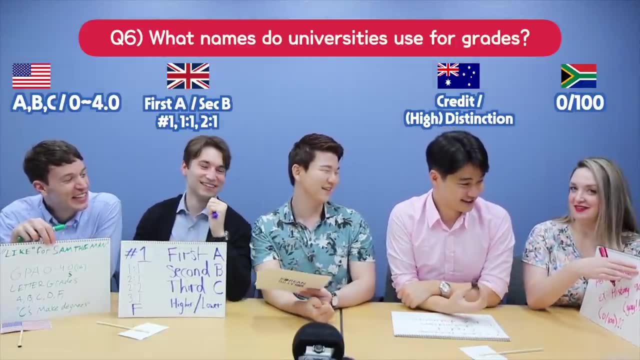 to our GPA With numbers. Yeah, But for each subject for the semester it would be something like this: I wasn't too much fun at university to pay much attention, but I was kind of competitive with points and scores and whatnot. 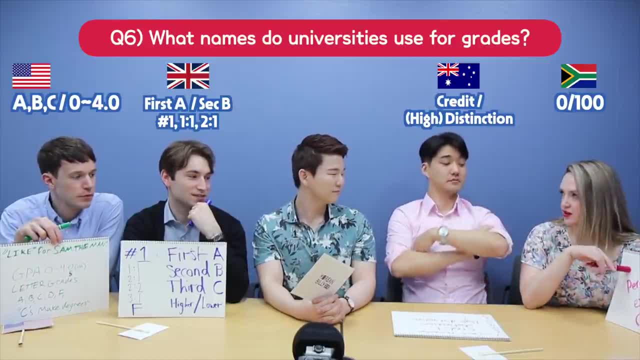 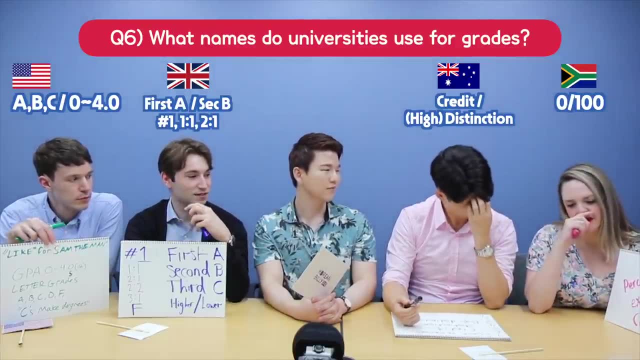 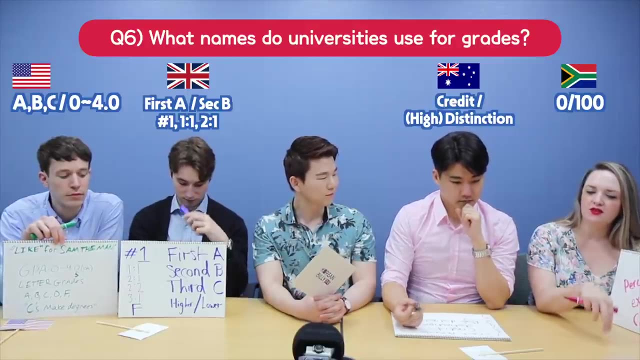 What I do remember at my universities it was mostly percentages. I remember looking at the report and whatnot, And then it would have like: history, you know 85%. or anthropology, you know percentage wise. Our ABCs was the final result of high school. 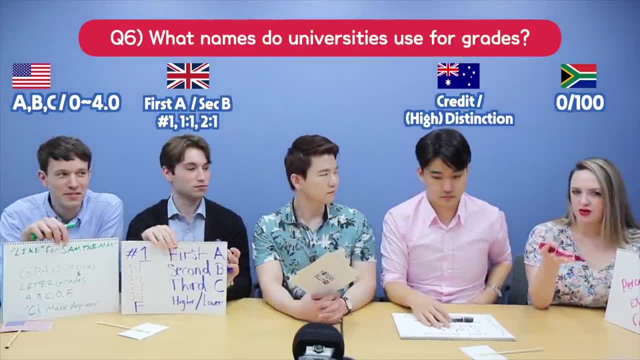 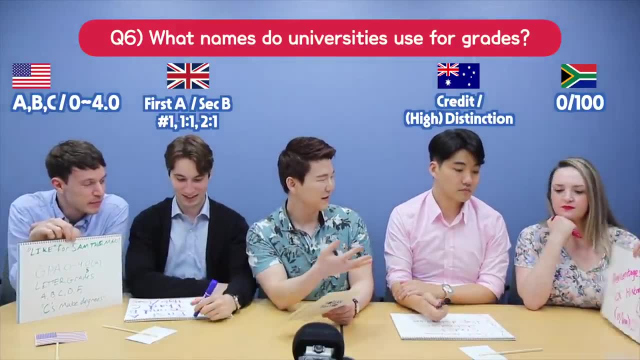 And then you'd see ABC. you know if you've got a distinction or whatnot, But from what I remember at university, it was mostly percentages to show what we got. Don't you use like GPAs, like 4.5, 4.0?? 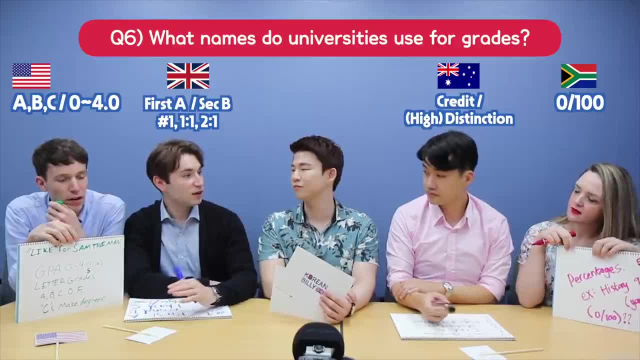 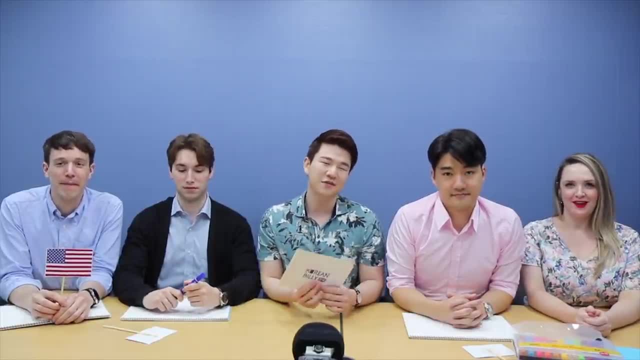 We don't use GPA too. We have to like convert everything Hmm To like a graduate school in a different country. All right, We've been taking a look at the educational system differences between US, UK, Australia and South Africa. Scoring systems are hard.